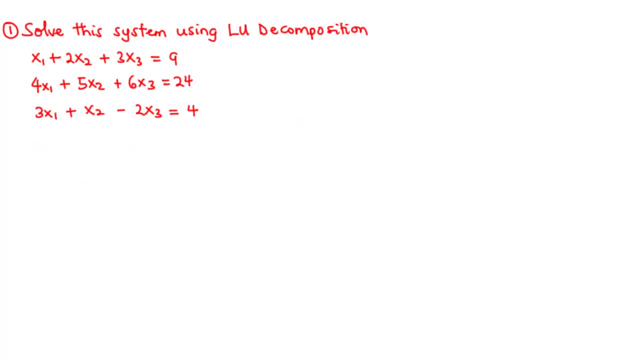 In this lesson we are going to learn how to solve a system of n linear equations with n unknowns using LU decomposition. Now, LU decomposition basically means lower upper decomposition. Let's try to solve this example together. So the first thing we are going to do here is to 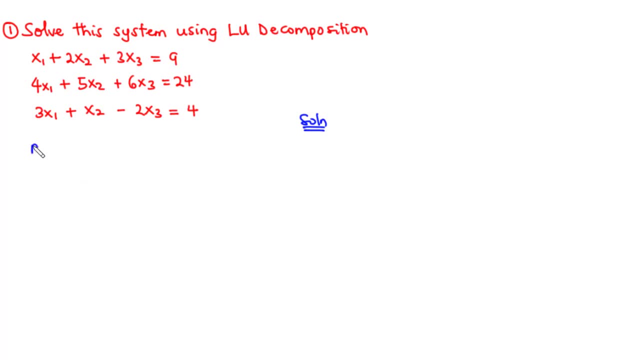 represent the system of linear equations in the form: ax equals b, where a is the coefficient matrix. x contains the unknown variables x1, x2, x3 and then b consists of the values that we see on the right hand side of each of the equations. Now the main idea is to decompose. 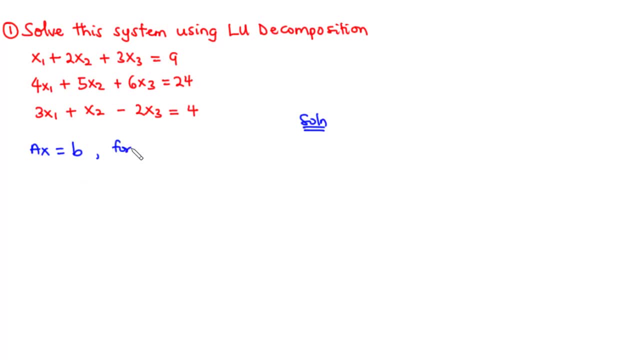 a into l times u, So we have for a equals l times u. we are going to substitute lu in place of a. Now we have a to be the coefficient matrix, and then we want to decompose this a so that we have a lower triangular matrix times an upper triangular matrix. So, considering this first, 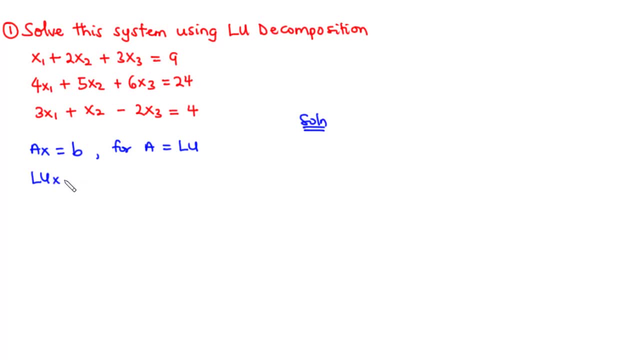 equation we are going to have lu times x, and that is equal to b. From this we can let ux be equal to z, so that if you substitute z in place of ux into this equation, then we have l times z equals b. So we call this equation one, and then 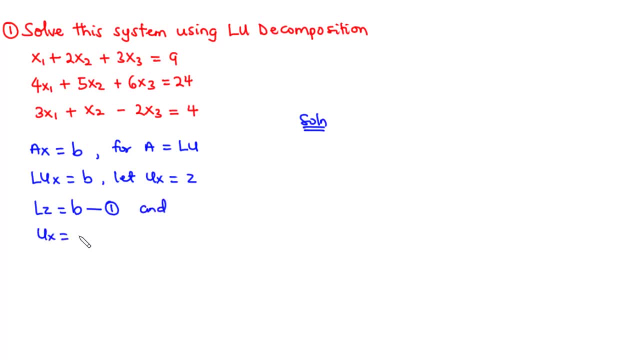 we have the second equation: ux equals z. So firstly we solve equation one for z, we substitute z into equation two and then we can solve for x. So basically, this is the procedure we are going to use to solve this system of linear equations using LU decomposition. So now let's begin the 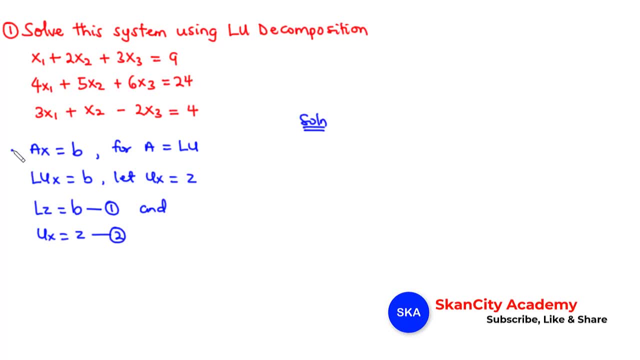 actual solution process. So first of all we are going to represent this system in the form: ax equals z, So we have the coefficient matrix, we have one, two, three, four, five, six, three, one negative, two times the color matrix, x. one x 2, x 3, and that is equal to values. on the right hand side we have 9, 24. 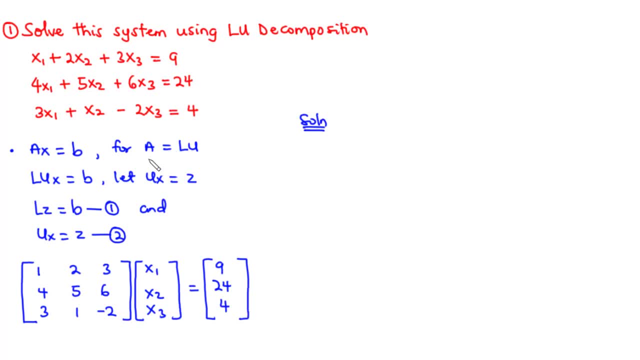 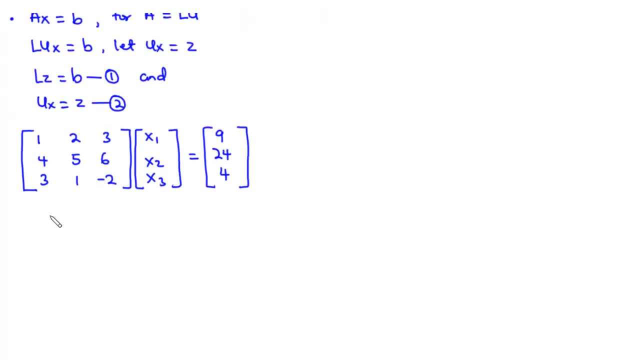 4. 9, 24, 4. 4. thing is we try to decompose a so that we have l times u. so we are going to have a is equal to. we have the lower triangular matrix. now we are going to make sure that the elements in the 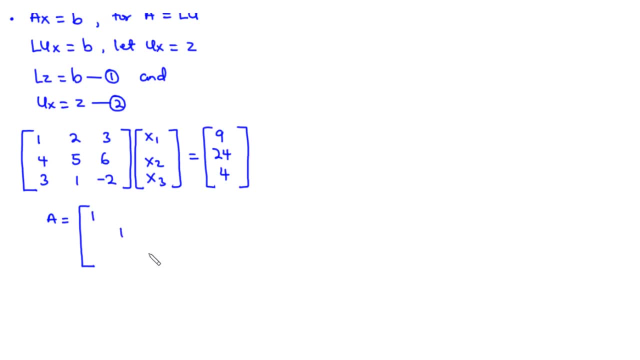 principal diagonal are all ones. elements above the principal diagonal are zeros. and then we have elements below the principal diagonal to be non-zero elements. now we call these elements multipliers, and these multipliers are the values that make the corresponding entries in the upper triangular matrix equal to zero. so we call these multipliers. we have the first one to be l two one. 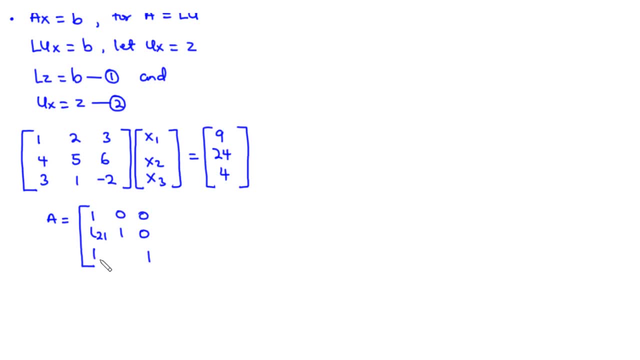 so, row two, column one, l three one, row three, column one, and then l three two, row three, column two. so this is the lower triangular, so this is the lower triangular, so this is the lower triangular matrix. this is l. and then we also note that these multipliers are basically called l values. 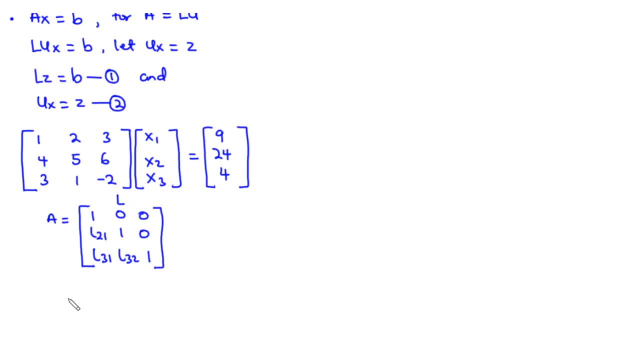 and to find these l values we need to find m values. so we say that the l values for the first one, l21, is equal to negative of m21, l31 is equal to negative of m31, and then l32 is equal to negative of m32. now, in the next moment, we are going to know how to find these m values. 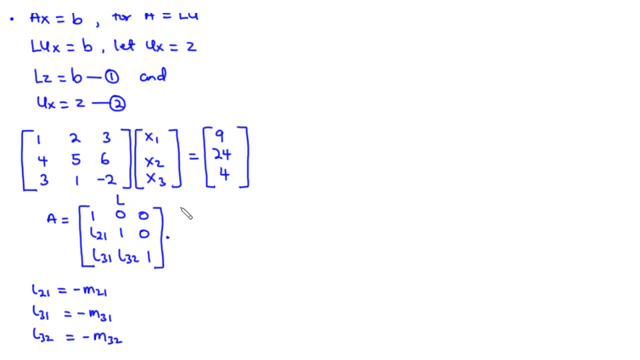 so we have the l parts times u so u. we have components u11, u12, u13, and then we have u22, u23 and then u33, and the elements below the principal diagonal are all zeros. so this is the upper triangular matrix. also notice that this upper triangular matrix is the same. 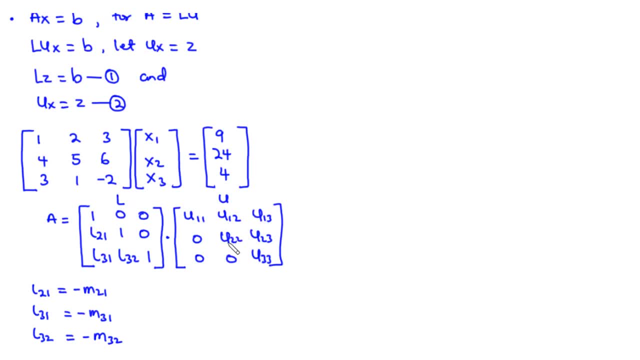 upper triangular matrix that is obtained at the end of the forward elimination steps of naive gaussian elimination method, which means that when you want to find the? u, the upper triangular matrix, you don't do any row swap. you don't do any row or column swap. so we are going to decompose. 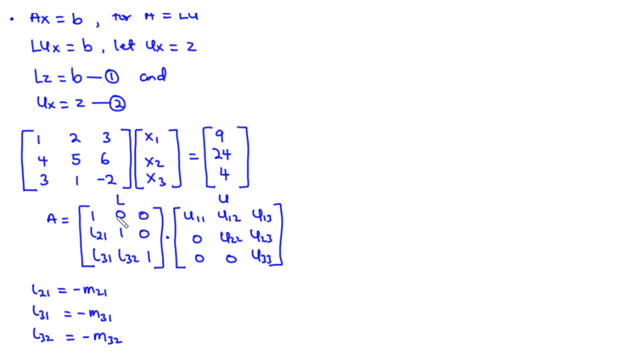 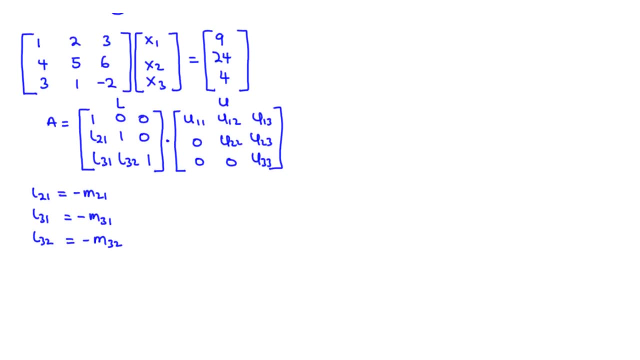 this coefficient matrix into a lower triangular matrix times an upper triangular matrix. So let's do that. So we have A to be 1,, 2,, 3,, 4,, 5, 6, 3, 1, negative 2.. Now the main idea here is to represent 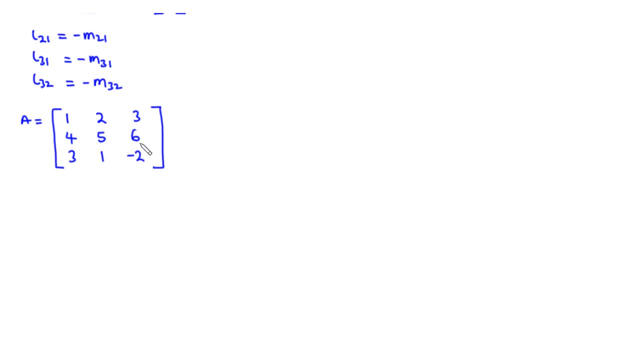 this as an upper triangular matrix. Now, in so doing we also obtain the multipliers to also form the lower triangular matrix. So at this point we are going to do forward elimination using naive Gaussian elimination method, which means that we are not going 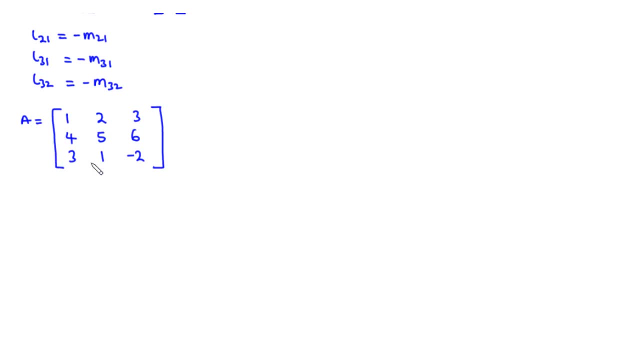 to do any row or column swap. Here we have three rows, so we are going to perform two forward elimination steps. In all, we want to make these three values go to zero. So in the first step we make these two values go to zero and then later we make this value. 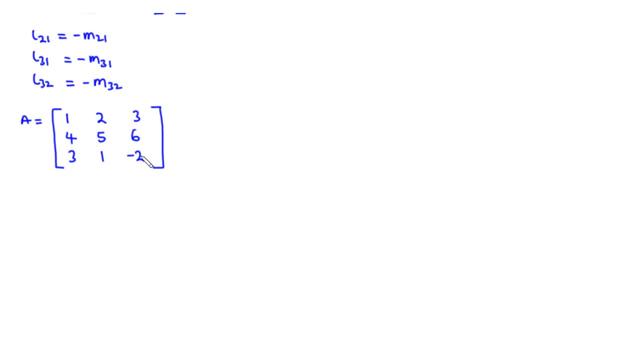 of 0.. So let's begin with the first forward elimination step. So we consider this to be the pivot row and thus want to be the pivot element. Now to make these two values go to zero, what do we do? We perform elementary row operations on row 2 and then row 3.. Now for row 2, to 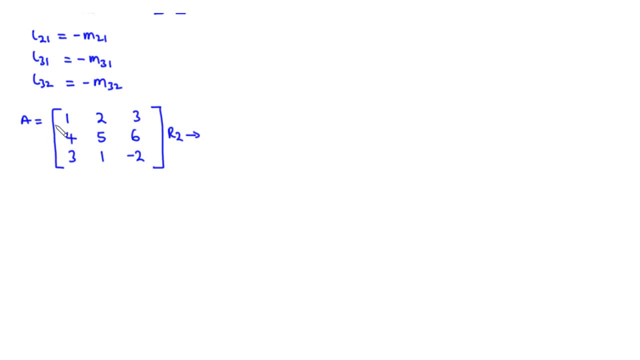 make this value go to zero. we are going to multiply row 1 by 4 over 1.. So 4 over 1 times row 1, and then we subtract the result from row 2.. If we do that for row 2, the first 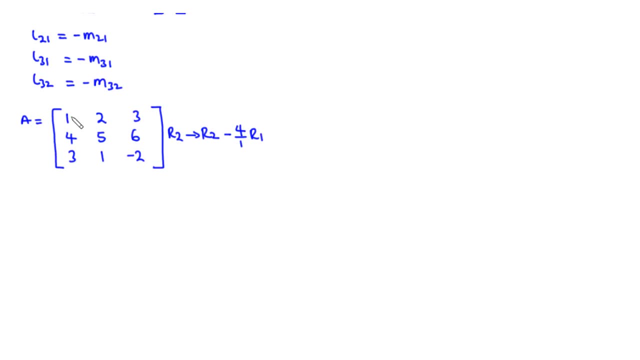 element we have 4, so 4 minus 4 over 1 times 1.. That goes to 0.. And then for row 3, we also perform elementary row operations. That's where we have we multiply row 1 by 3 over. 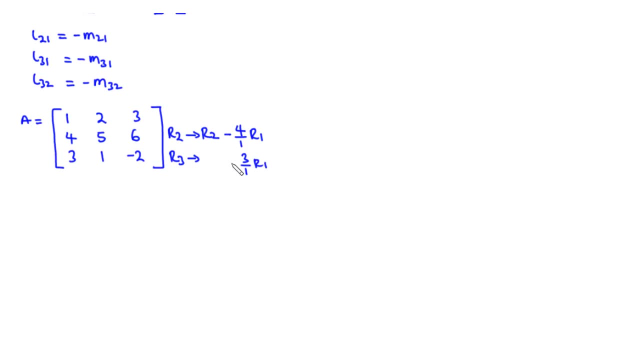 1, so we have 3 over 1 times row 1.. We subtract that from row 3.. First element of row 3 is 3.. 3 minus 3 over 1 times 1 is 0. And so from row 2, we have, we have a loop to the left. 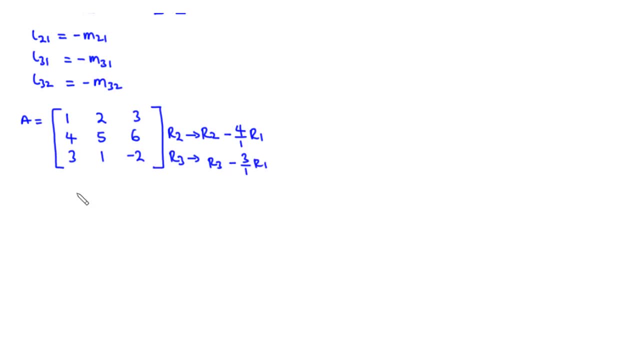 which is equal to 2 over 0. And then, in the form below, we have relatively simple HTML fals. So we have, we have alpha over 1 and then eventually subtract R0.. Made at the first point one is zero, so let's perform the operation. actually, row one remains the same, so we have one. 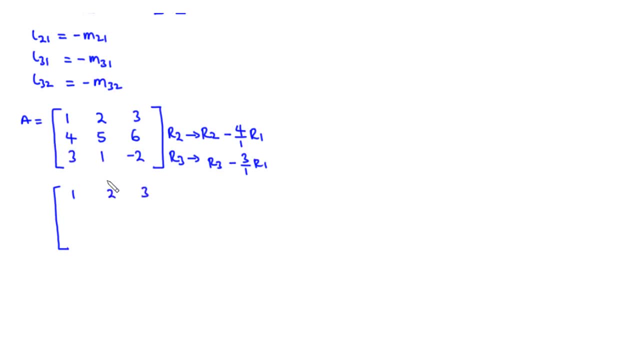 two, three and then for row two, we have first element four minus four over one times one. that is zero. and then we move on to column two. we have five minus four over one times two. that becomes negative. three to column three: we have six minus four over one times three. that becomes negative. 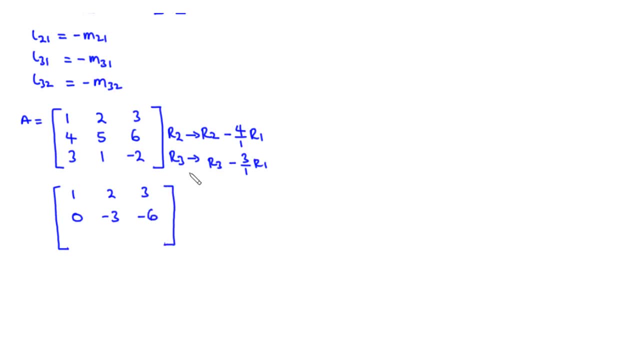 six, we move on to row three. row three, first element: we have three minus three over one times one, that is zero. column two: we have one minus three over one times two, that becomes negative five. and then we have column three, negative two minus three over one times three, and that also. 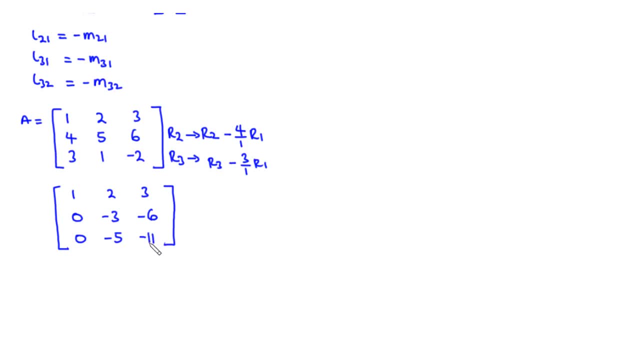 becomes negative three. and then we have column three negative two minus three over one times three, and that also becomes negative three minus three over one times three over one times three. so we succeeded in making these two values go to zero. now let's move on to the second forward elimination step. we want to 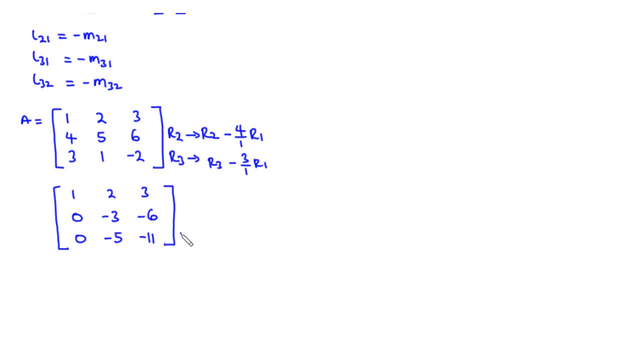 make this value go to zero. so what we do? we perform elementary operations on row three. and what is the operation? we are going to multiply row two, because this time row two becomes the pivot rule and then negative three becomes the pivot element. so we multiply row two by negative five. 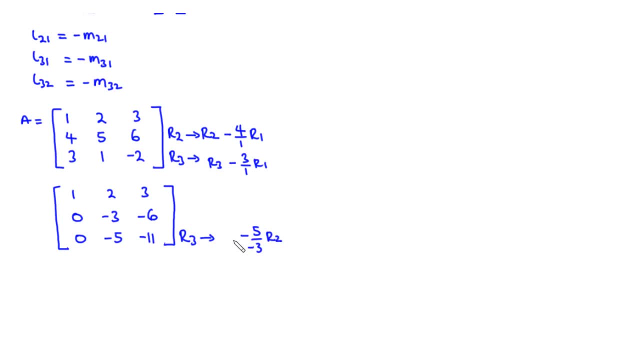 over negative 3, and then we subtract the results from row 3.. Now negative cancels out negative, so we can simply write this as row 3 minus 5 over 3 times row 2.. So row 1 and then row 2 remains the same. 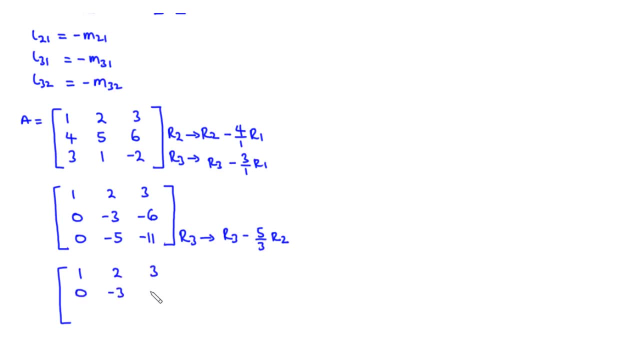 and then for row 3, we have 0 minus 5 over 3 times 0, that is 0.. We have negative 5 minus 5 over 3 times negative 3, that is also 0. and then, lastly, we have negative 11 minus 5 over 3 times negative 6. 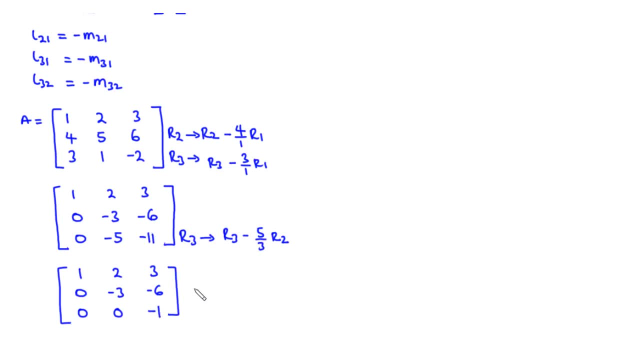 and that is negative 1.. So basically this is the upper triangular matrix which you obtain after forward elimination steps. Now we are going to write down the multipliers. So for the multipliers, the first one is we have m2 1.. Now for m2 1, that is going to be the coefficient of r1 here. 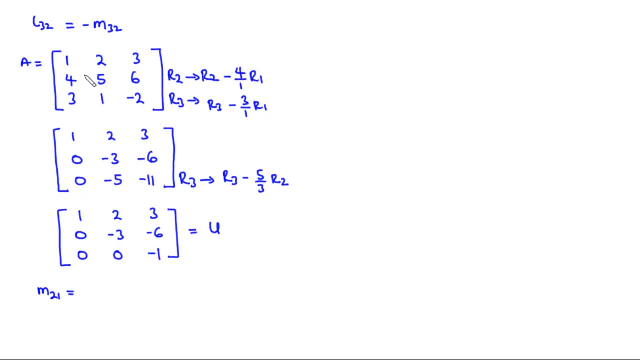 because this is the value that makes this value go to 0. So we are going to have negative 4, that is, m2 1.. Now we are going to write down the multipliers. So for the multipliers, we are going to have negative 4.. Similarly, m3 1, we are going to have negative 3. 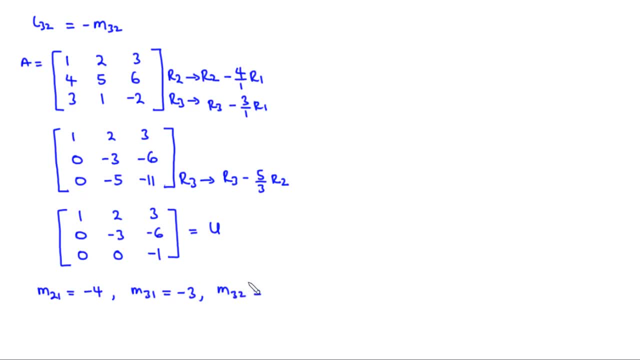 and lastly, m3 2, we are going to have negative 5 over 3.. Now, since the l values are basically opposite of the m values, we are going to have the opposite of negative 4 to be 4.. So we can simply write negative 1 times negative 4, and then we have 4, and then we move on to. 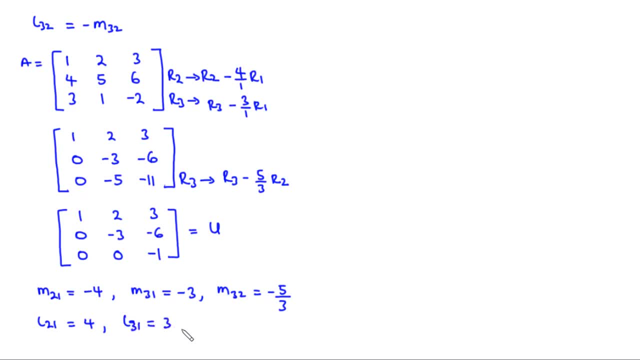 l31, that is equal to 3, and then l32, that is equal to 5 over 3.. So basically, these are the l values we are going to put in the l matrix. So we are going to have l also being equal to. We have 1, 1, 1 in the principal diagonal, 0, 0, 0 here. 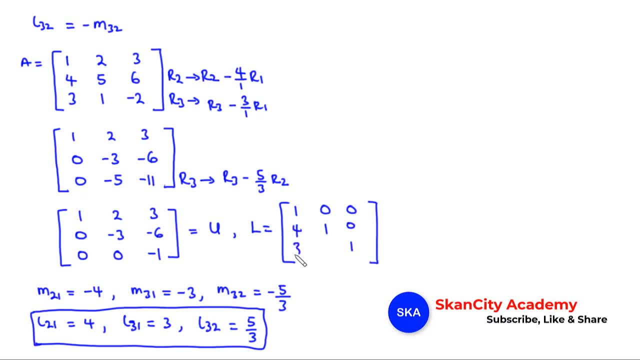 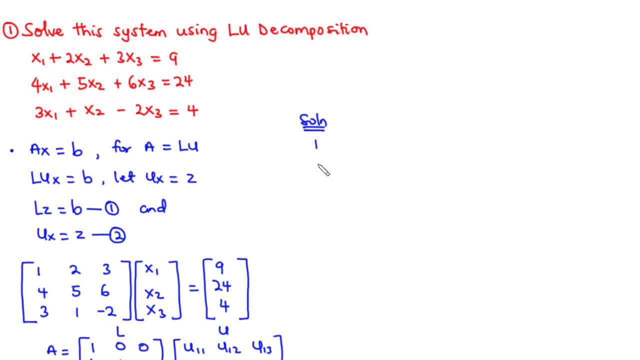 And then we are going to have 4,, 3, 5 over 3.. So primarily, what this means is that we've been able to decompose this coefficient matrix- 1,, 2,, 3,, 4,, 5,, 6,, 3, 1, negative 2- into a lower triangular matrix having components or having elements. 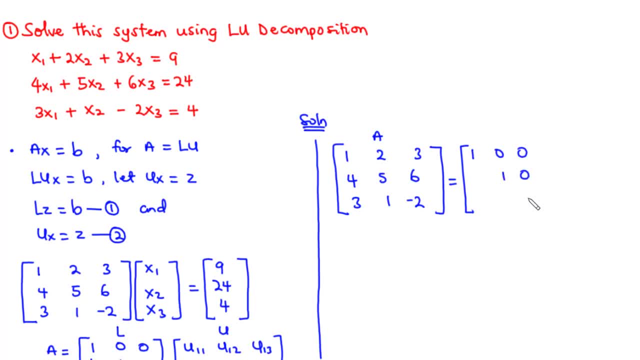 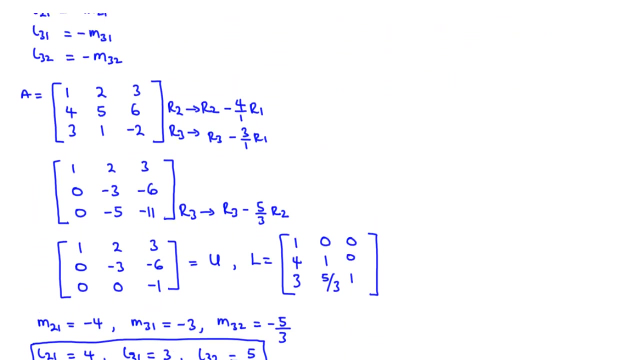 1, 0, 0, 1, 0, 1,, 4,, 3, 5 over 3.. Times an upper triangle Triangular matrix of elements 1,, 2,, 3, negative, 3, negative, 6, negative, 1.. 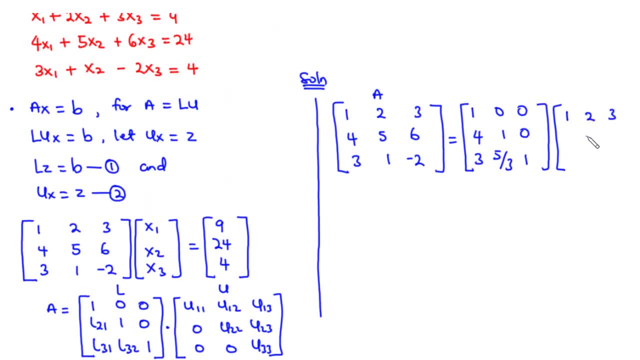 So 1,, 2,, 3, negative, 3, negative, 6, negative, 1.. And then here we have 0, 0, 0.. So this is L times U. Now, after doing this, we need to solve. 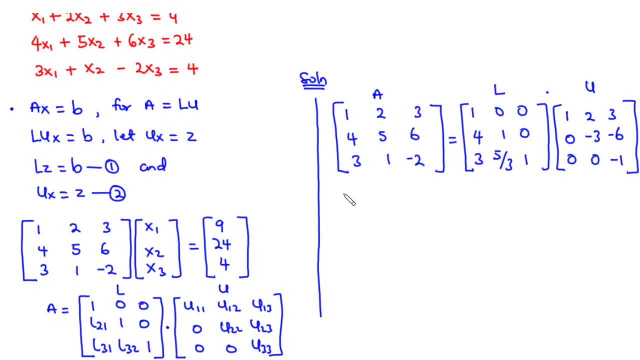 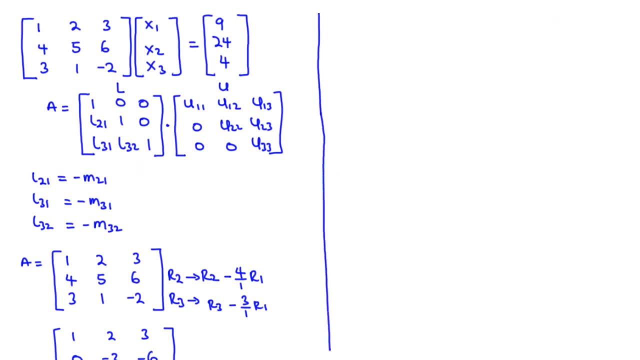 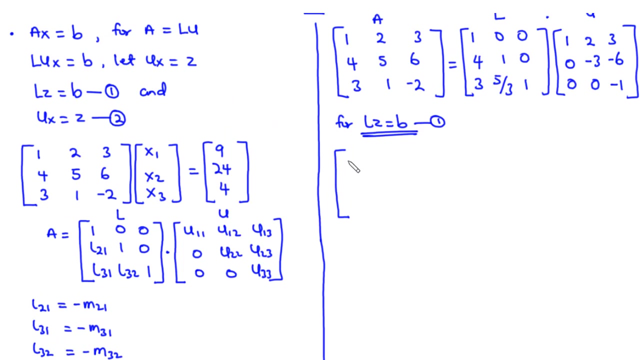 We need to solve for Z using equation 1.. So for LZ equals B, that is equation 1, we are going to solve for Z. So we have L, which has elements 1, 0, 0, 4, 1, 0. 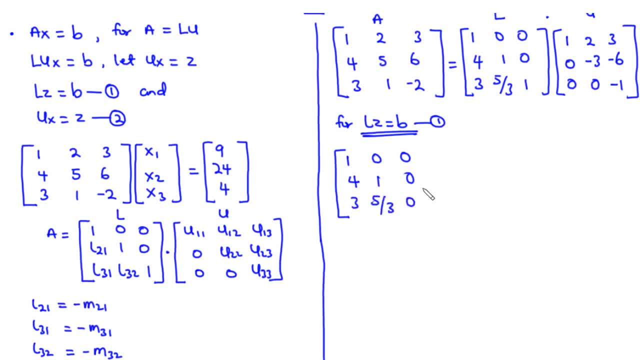 3, 5 over 3, 1. Times we have the Z values to be Z1, Z2, Z3.. Equal to B, 9,, 24, 4.. So here we are going to do forward substitution. 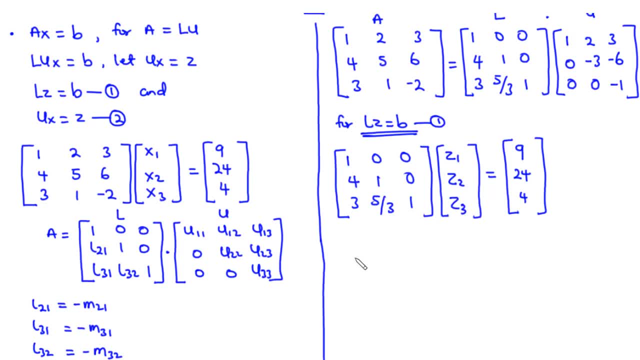 Here we are going to do forward substitution. So here we are going to do forward substitution: the values of z1, z2 and then z3. so for the first one, we consider row 1, we have 1 times z1, 0 times z2, 0 times z3. notice that column 1 corresponds to z1. 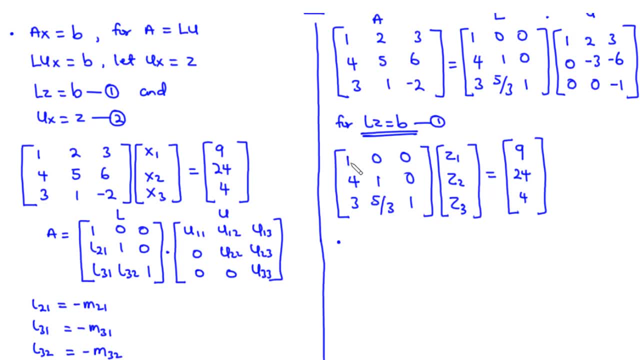 column 2: z2. column 3: z3. so we have 1 times z1, that is z1 equals 9, because we are going to have 0 times z2, which is 0, plus 0 times z3, which is also 0, so we 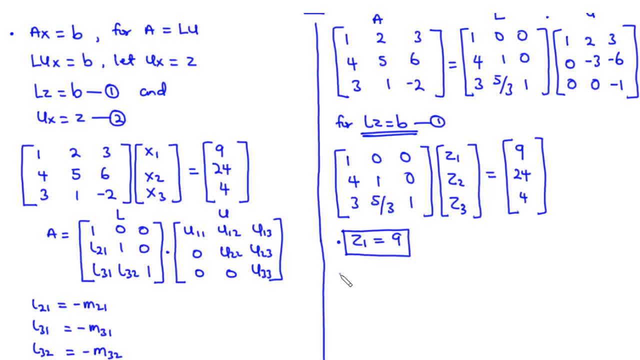 have. z1 equals nine. now let's move on to row 2. so for row 2, we are basically going to have four times z1, which is 4 times 9, plus 1 times z2, so we have z2 0 times z3, which is zero, so this is equal to 24. so you are going to have 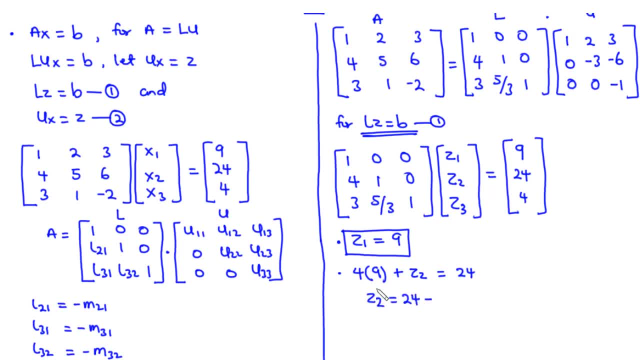 z2 equals z3: 0, 0, 1, 1, 1, 24 minus. we transpose this to the right hand side: 4 times 9 is 36, so we have z2 to be equal to negative 12.. now let's move on to row 3. that's where we have 3 times z1. z1 is 9 plus 5 over 3. 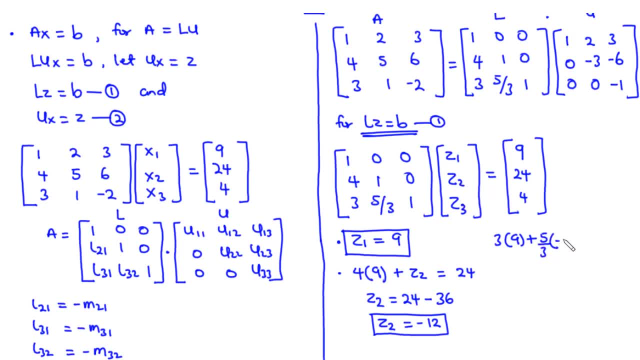 times z2, which is also negative, 12, and then plus 1 times z3, which is z3 equals 4, so here 3 goes here once. 3 goes here 4 times 3 times 9, that is 27, 5 times negative, 4, negative, 20 plus z3. 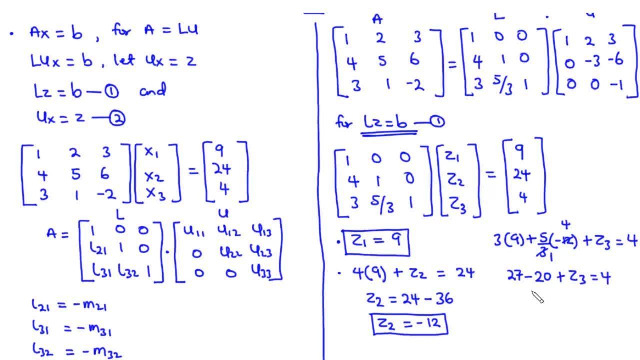 equals 4. so here we have 7 plus z3 equals 4. we transpose 7 to the right hand side, that is 4 minus 7 and that is equal to negative 3, negative 3. so we have z3 to be equal to negative 3. now these are z values we are going to substitute. 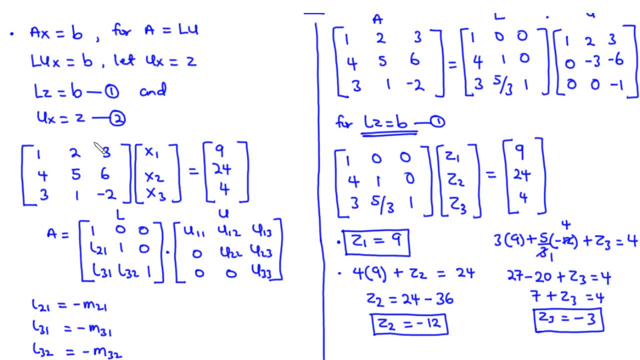 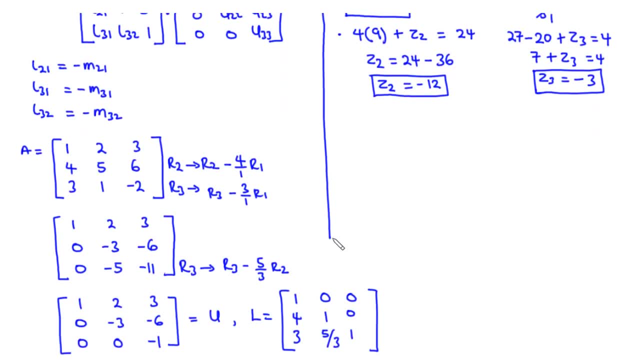 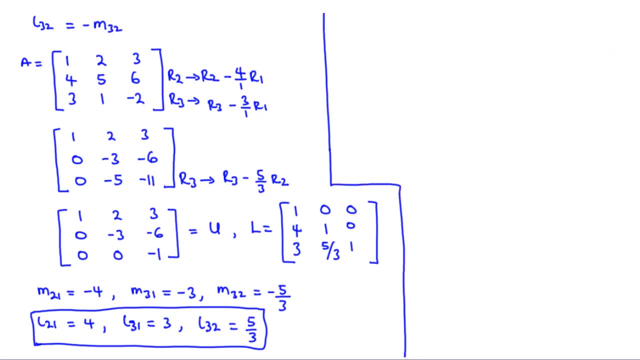 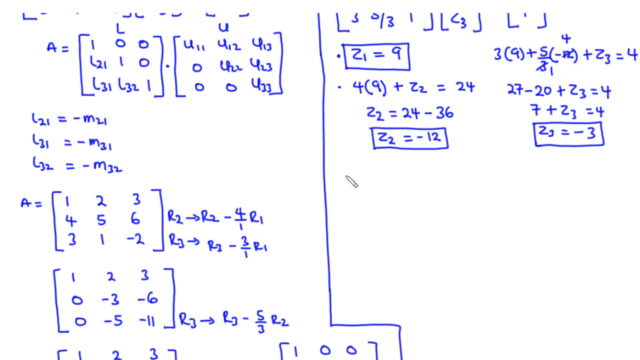 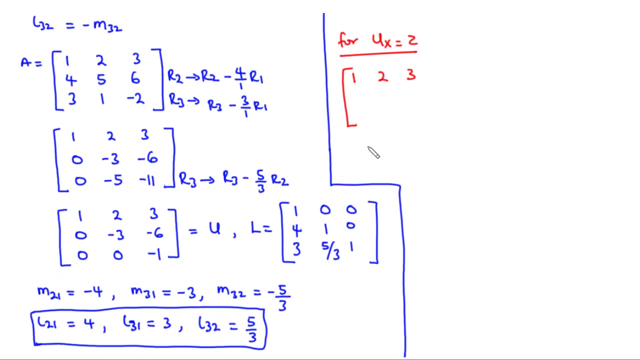 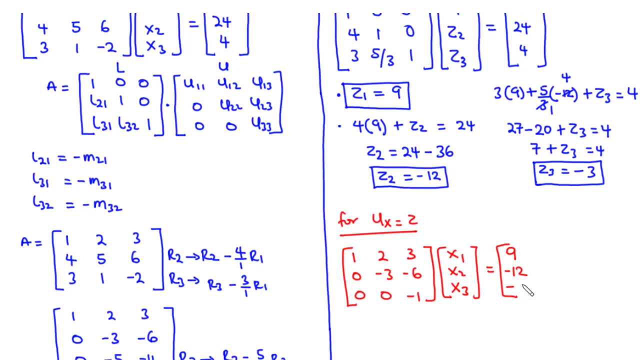 these z values into equation 2. so let's move on to equation 2. so for equation 2, that is ux equals z, so we have the upper triangular matrix, which is, which is ux equals z. so we have z1 to be 9, z2 negative, 12, z3 negative 3. so let's try to find the values of. 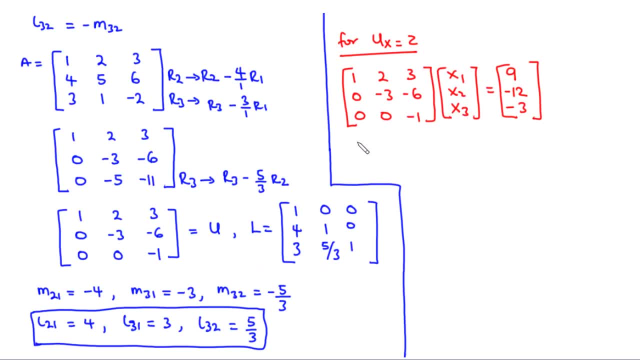 x1, x2, x3. so here we are going to do back substitution. so we have negative 1 times x3. so negative x3 equals negative3. therefore we divide through by negative 1, negative 1, and then we have x3 to be equal to 3. next we move on to row 2, so we have 0 times x1, that is, zero negative. 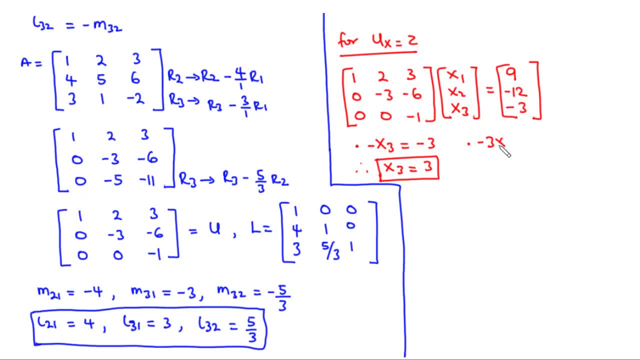 3 times x2, so negative 3x2. so we'll be using 0, x1, x2, 2 and then minus 6 times x. 3 x 3 is 3, that is equal to negative 12. so here we are going to have. 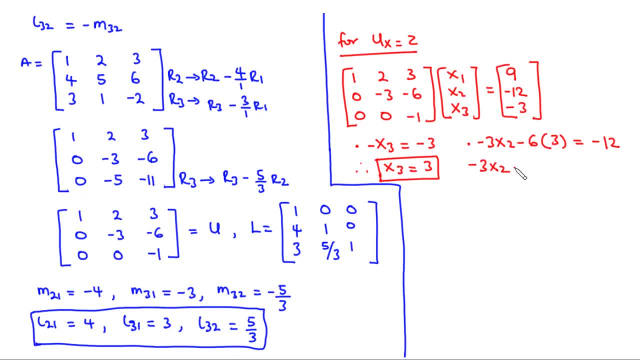 negative 3 x 2 minus 18 equals negative 12. so we have: negative 3 x 2 equals negative 12 plus 18, which is equal to 6. we divide through by negative 3, by negative 3, and then we have x 2 to be equal to negative 2. so this is the value of x 2, and then we move on to row 1. we have: 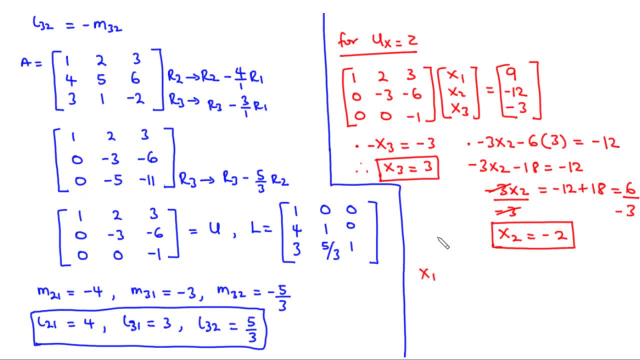 x 1, so 1 times x 1 is x 1 plus 2 times x 2, which is negative, 2 plus 3 times x3, which is 3, and that is equal to 9. so we have x1 minus 4 plus 9 equals 9. 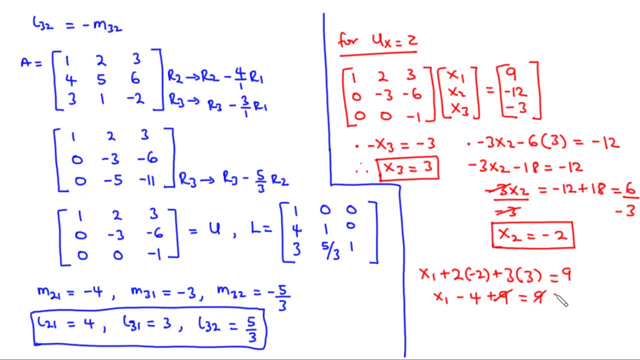 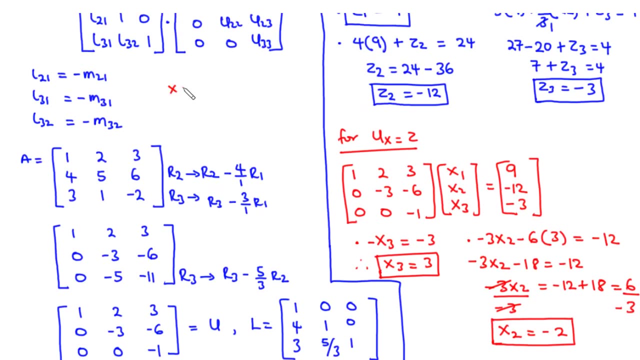 so 9 cancels out 9. we are left with 0. here, therefore, we have x1 equals 4. therefore. therefore, we have the solution vector x to be equal to the column matrix x1, x2, x3, and that is equal to. we have x1 to be 4. 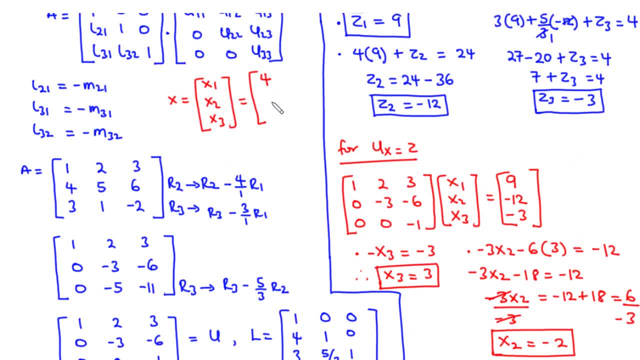 x1 is 4, x2 negative 2, x3 and that is equal to 3.